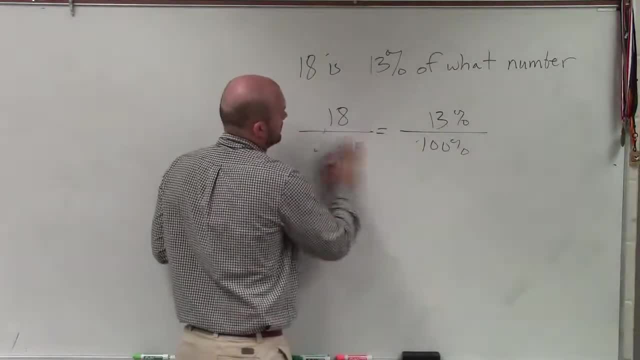 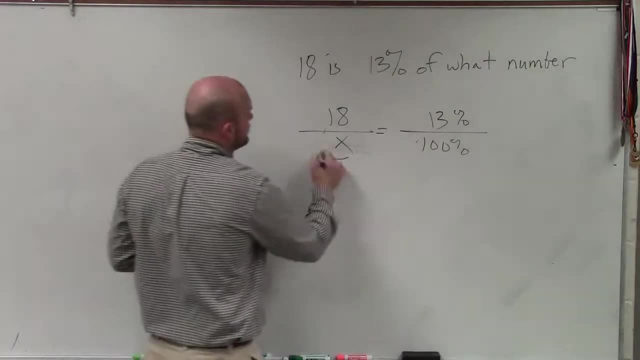 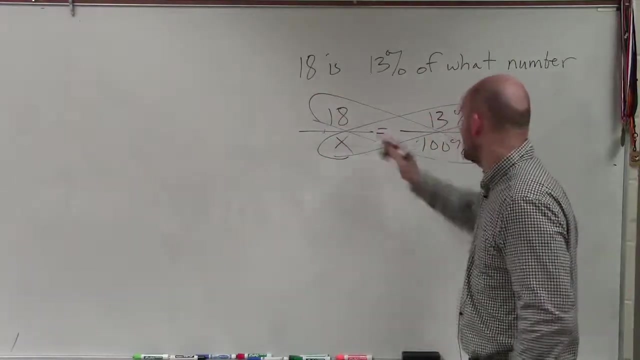 did a problem where it's the whole, So we'll have X be our whole. So again, what we can look at, Taylor is again applying cross multiplication, All right, And getting back to this again, we have 18 times 100%. 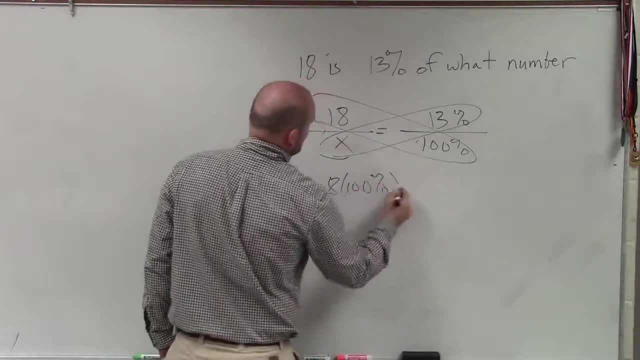 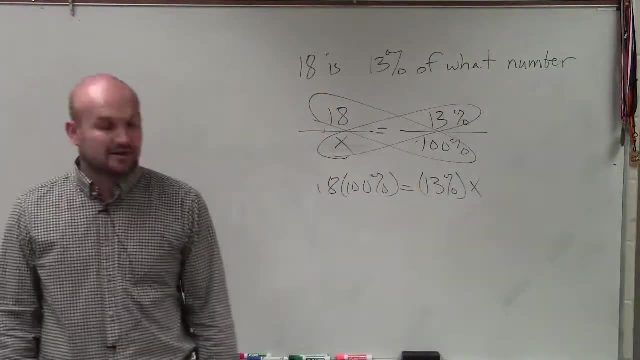 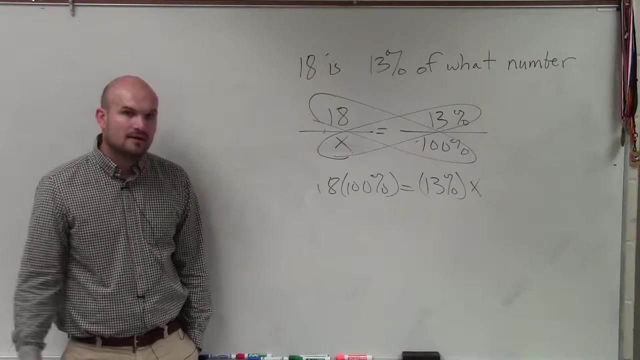 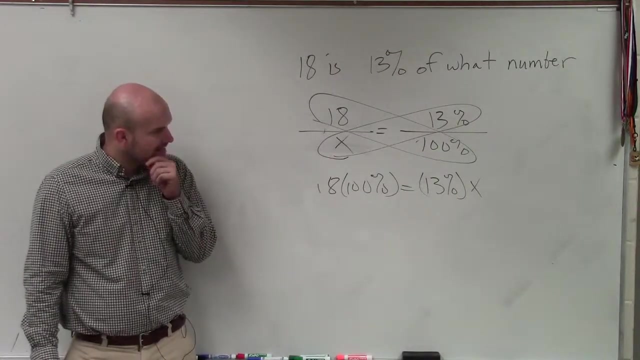 is equal to 13% times X. Now, ladies and gentlemen, again there's multiple different ways that you could go about this. all right, as far as dealing with the percentages or not. I mean, multiplying it with all those zeros is not going to be that bad, But I think what is easier is just 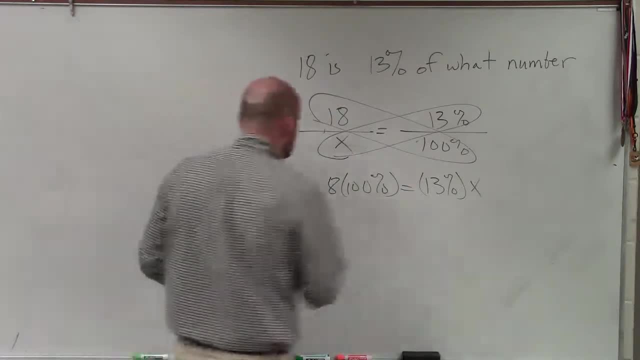 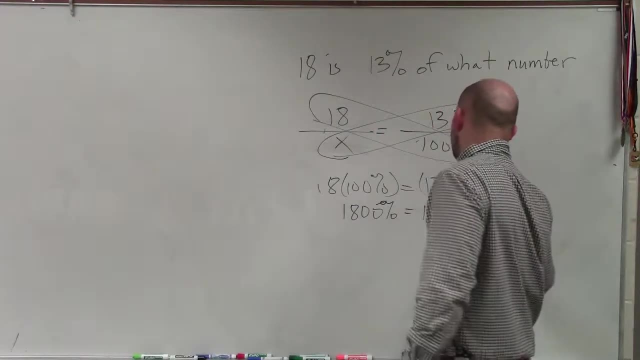 to divide everything. Actually, never mind, It's not going to matter, It's going to be the same thing. So let's multiply this to 1,800% equals 13% X, And again we want to figure out the whole. 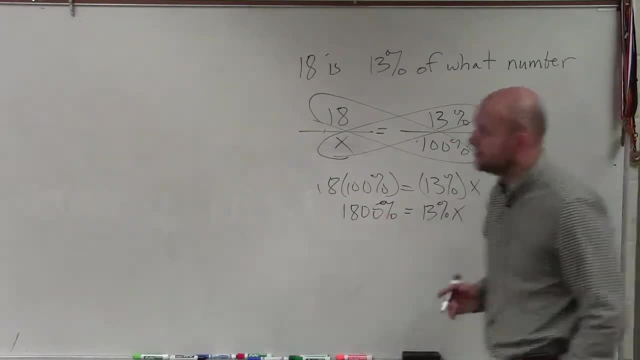 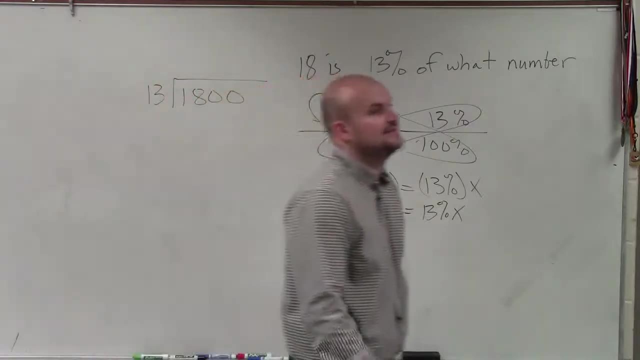 So I need to now divide 13 into 1,800.. So let's go back to our long division. All right, How many times does 13 go into 1,800?? Well, 13 doesn't go over to 1.. So we go to 18.. 13 goes into. 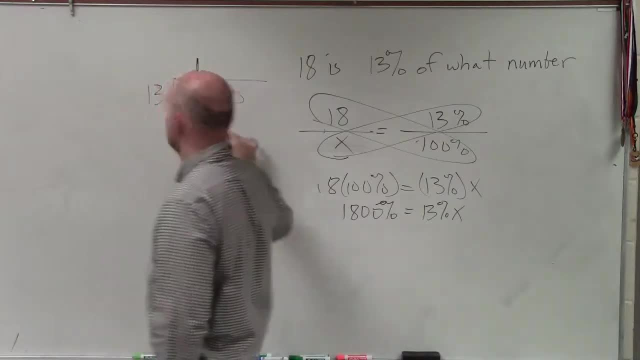 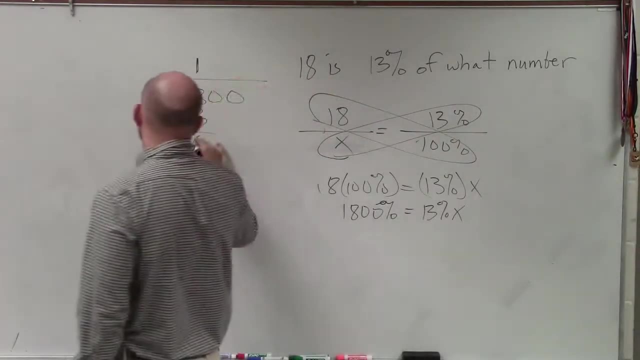 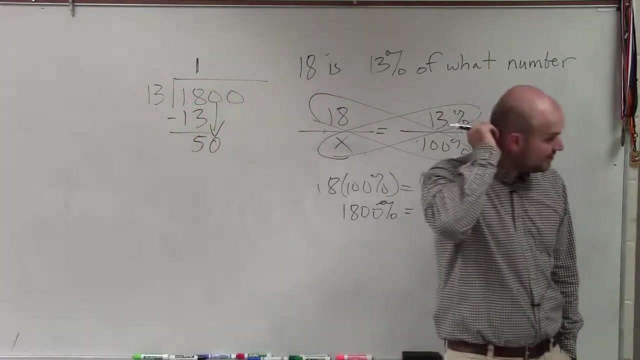 18 one time. 1 times 13 is 13.. Sorry, Then we subtract 18 from 13,, which is going to give us 5.. 13 does not divide into 5. So we bring down the next zero, But 13 does go into 50. And it goes. 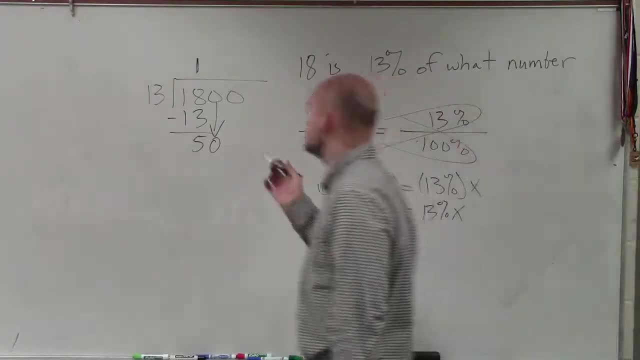 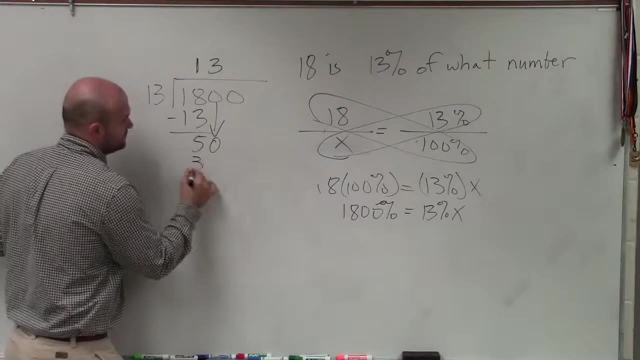 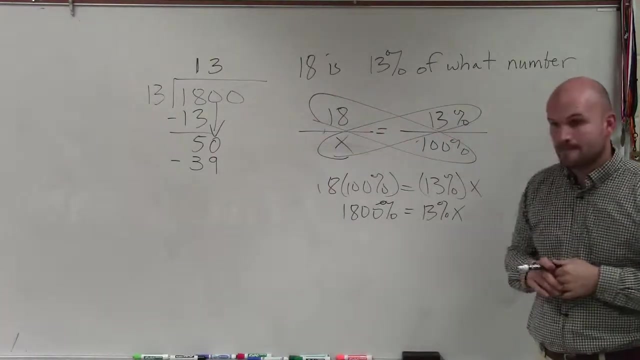 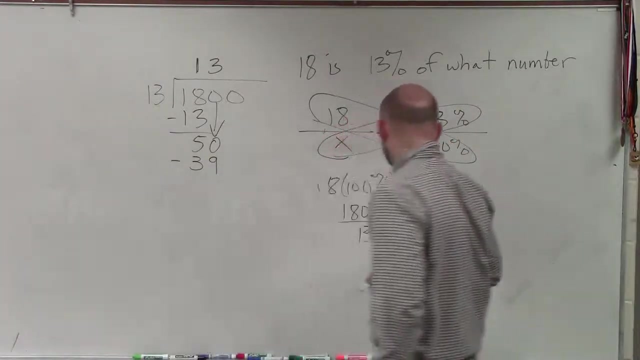 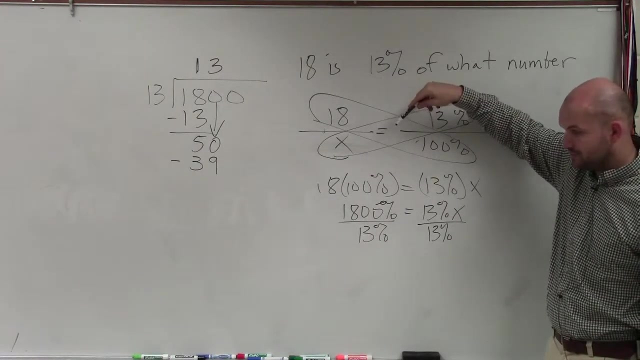 into there: 26, three times 3.. 3 times 13 is going to be 39.. Wait a minute, What You lost. Where did I lose you? So all I'm doing is again, as long as I can have you from here. you've set up the proportion. apply the. cross product. 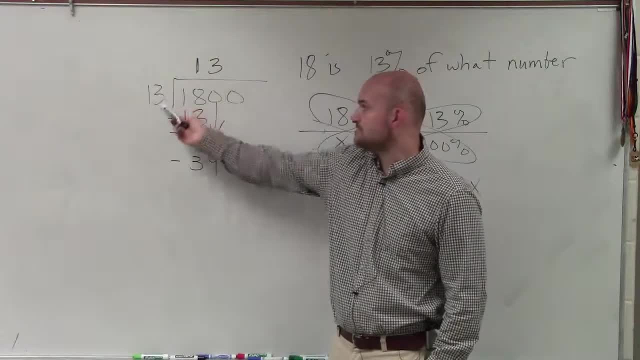 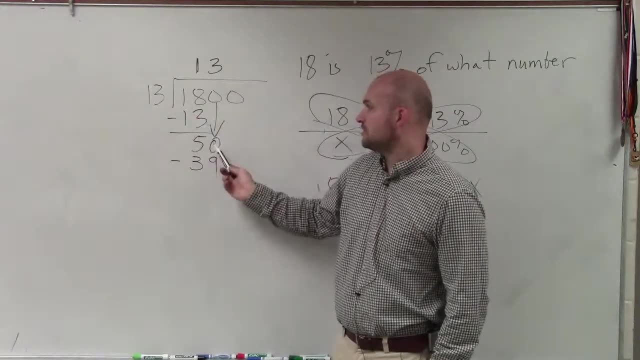 1. 13 goes into 18. one time 1 times 13 is 13.. 18 minus 13 is 5.. 13 does not go into 5, so I brought back the 0.. 13 goes into 50. three times 3 times 13 is 39.. Subtract them.